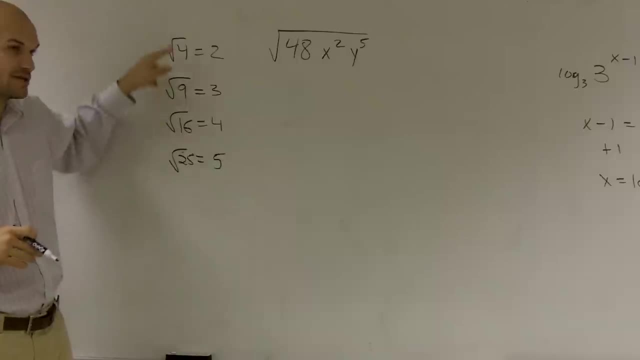 is: we want to try to get these numbers. we want to re-represent this problem by only using these numbers. Okay, because we can take the square root of this. So what I'm going to do is: I want to see: can I transform the square root of 48 by using these numbers? 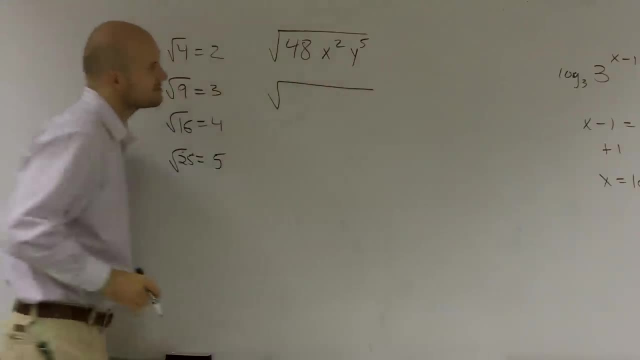 Rewrite it And what we can look at this and say, well is, can I use and you can say like factor it, can you kind of break down the factor 48 as using as the multiple of one of these numbers? 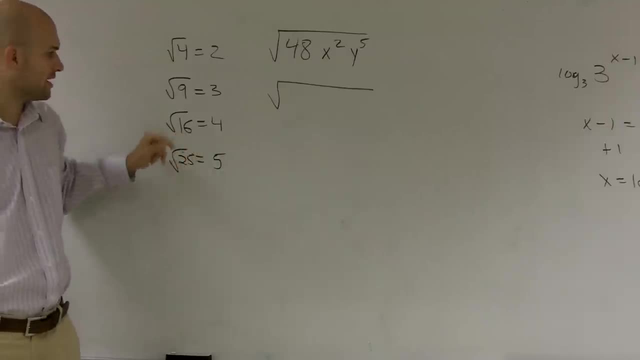 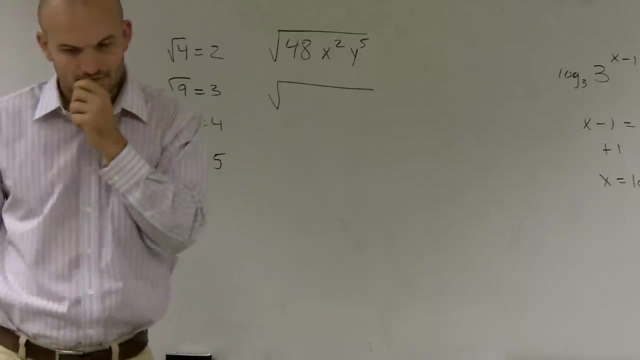 And the answer is Yes. Yes, you could write it as what? 4 and 12.. You could write it as 4 and 12.. I would say you could write it as 4 and 12,, which is not wrong. 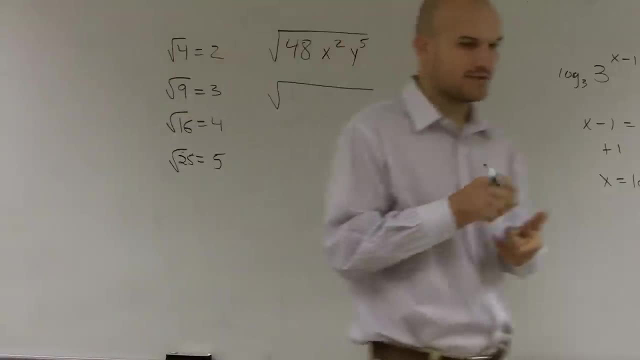 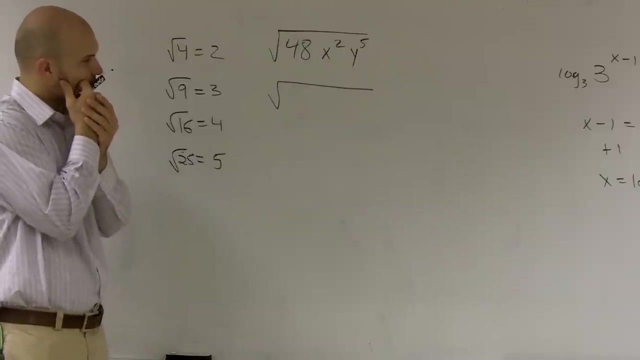 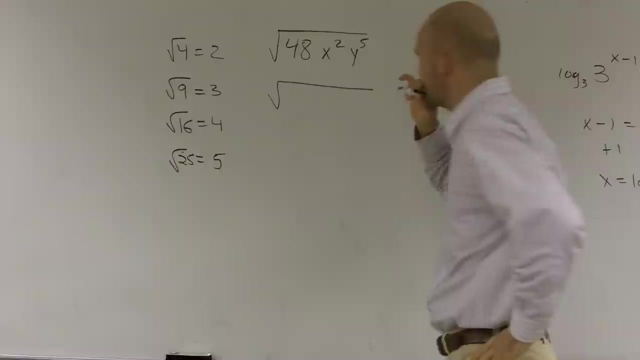 But you want to. if you do it as 4 and 12, the thing that's going to be tough is you can always you're going to have to simplify it again, So it's um, well, okay, so let's try it. 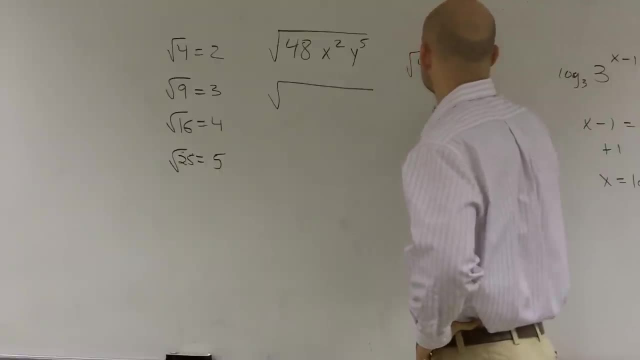 So you guys had 4 times 12, right, 6 times 8, 24 times 2,, 16 times 3.. Those are our three out. Those are Those are our options. right, You could obviously do 48 times 1 and stuff like that, but that wouldn't change it. 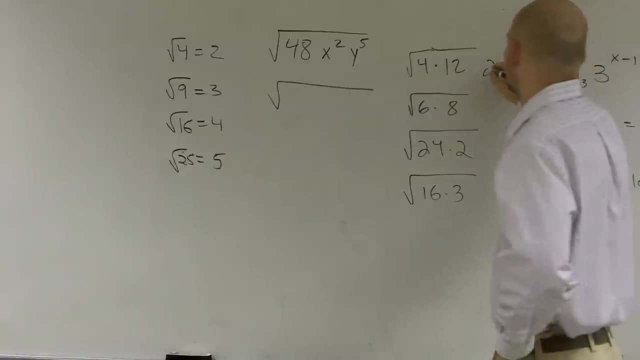 Well, let's look at it this way: You could rewrite this as 2 times the square root of 12.. The square root of 4, we know, is 2, right Yeah, 12.. Can I take the square root of either one of these numbers? 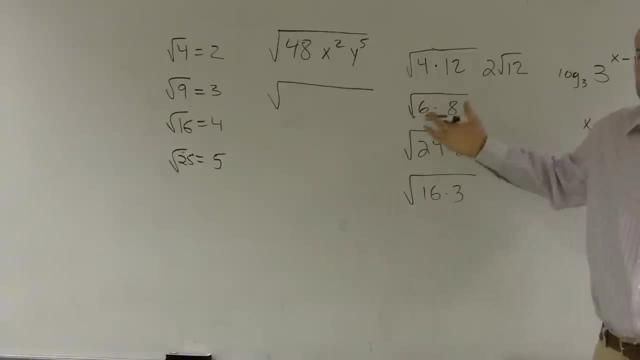 No right, So I can't. you wouldn't want to choose 6 and 8, because you can't take the square root of any of them Here. um, I can't take the square root of 24, nor can I take the square root of 2.. 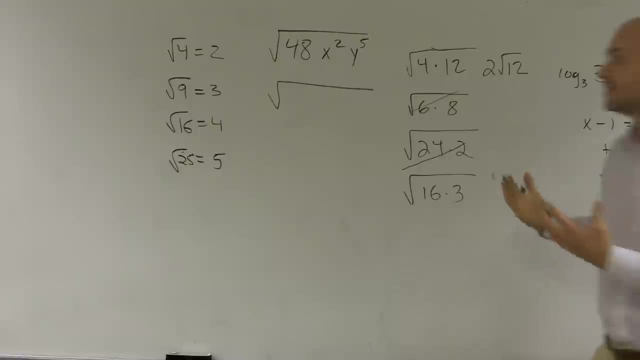 So again, this one you would not want to choose again because you can't remember. our whole goal is, it says, to simplify the radical. That means I need to see what numbers can I take the square root of. So so far we only have 1 we can take the square root of, and that was 4 times um the square. 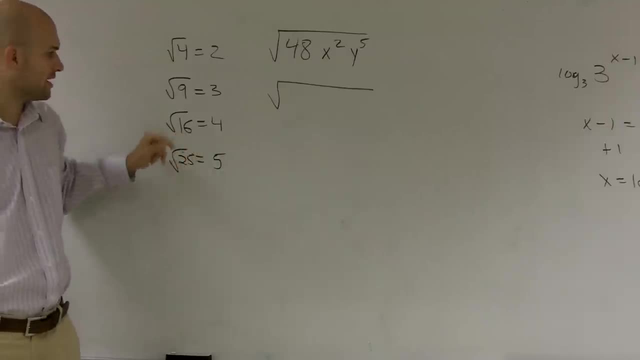 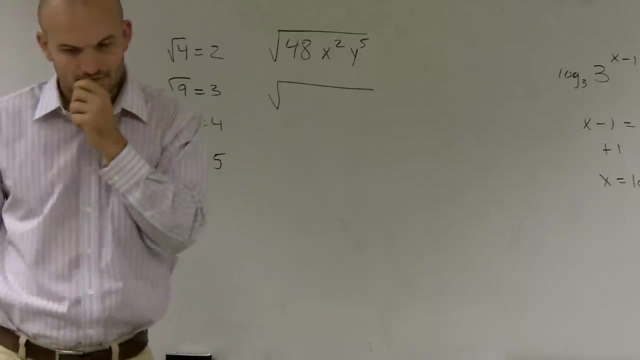 And the answer is Yes. Yes, you could write it as what? 4 and 12.. You could write it as 4 and 12.. I would say you could write it as 4 and 12,, which is not wrong. 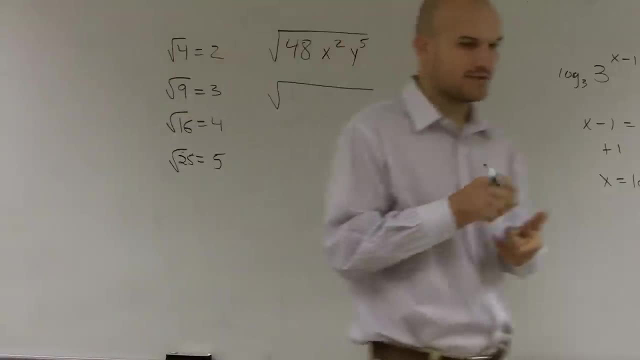 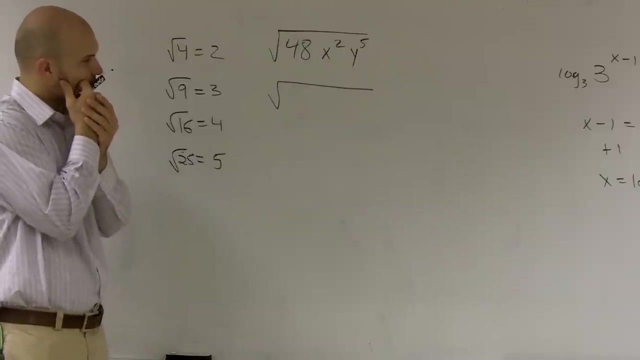 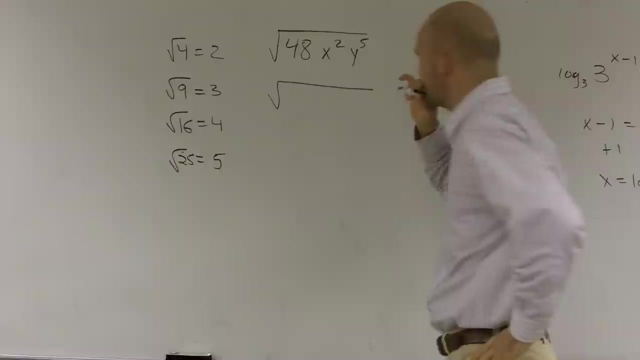 But you want to. if you do it as 4 and 12, the thing that's going to be tough is you can always you're going to have to simplify it again, So it's um, well, okay, so let's try it. 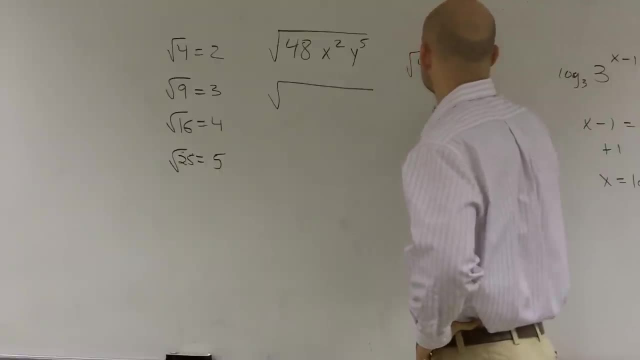 So you guys had 4 times 12, right, 6 times 8, 24 times 2,, 16 times 3.. Those are our three out. Those are Those are our options. right, You could obviously do 48 times 1 and stuff like that, but that wouldn't change it. 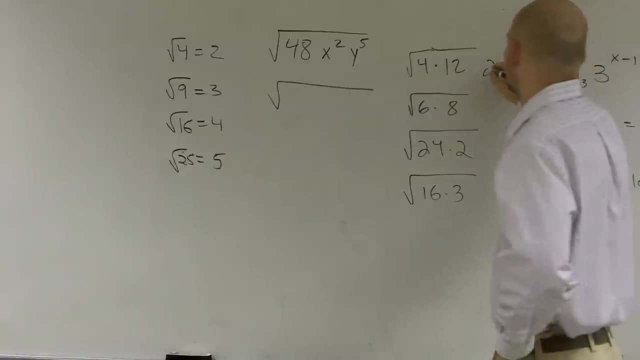 Well, let's look at it this way: You could rewrite this as 2 times the square root of 12.. The square root of 4, we know, is 2, right Yeah, 12.. Can I take the square root of either one of these numbers? 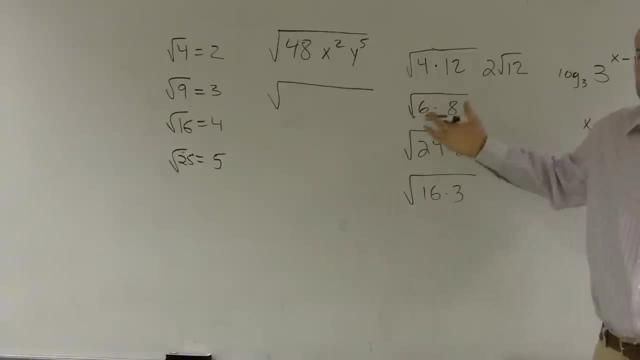 No right, So I can't. you wouldn't want to choose 6 and 8, because you can't take the square root of any of them Here. um, I can't take the square root of 24, nor can I take the square root of 2.. 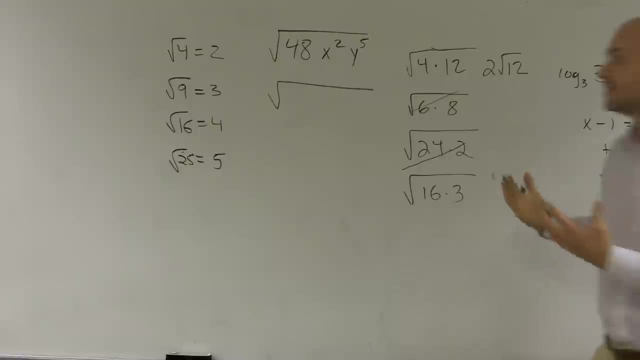 So again, this one you would not want to choose again because you can't remember. our whole goal is, it says, to simplify the radical. That means I need to see what numbers can I take the square root of. So so far we only have 1 we can take the square root of, and that was 4 times um the square. 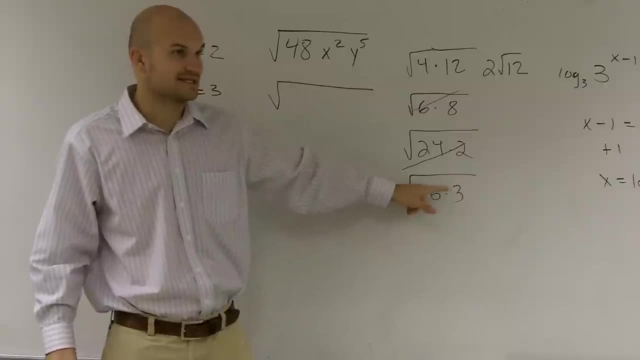 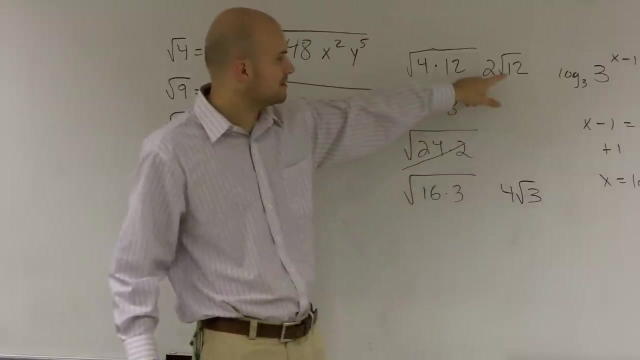 root of 12.. Or you could also choose 16 times 3, can you take the square root of 16?? Yeah, Yes, It's 4 times radical 3.. Now the reason why I didn't- um, I said I wouldn't choose this one. there's nothing. 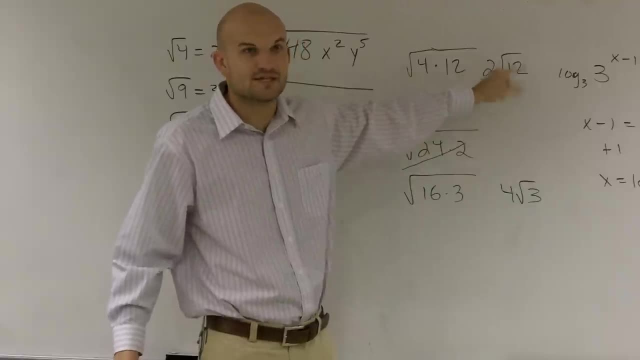 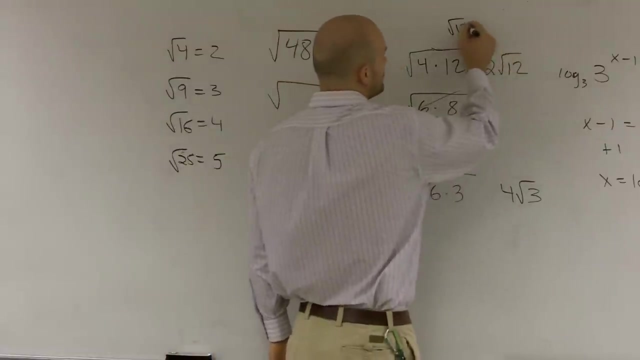 wrong with this one. But what you notice is: you can do this, you can simplify this one again. So it's not wrong, it's just you need to simplify it again. So square root: now you can do square root of 12, can reduce down to 4 times square root. 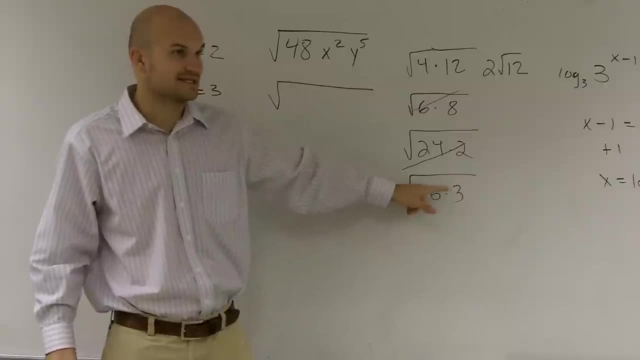 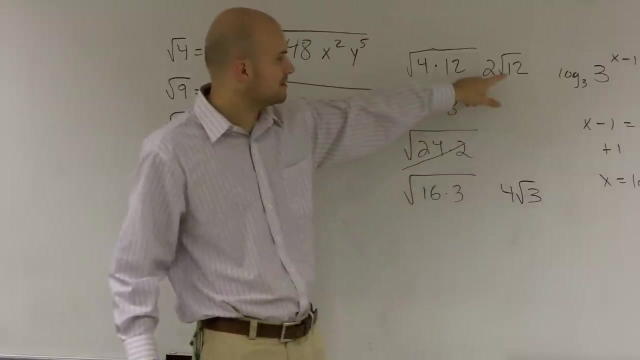 root of 12.. Or you could also choose 16 times 3, can you take the square root of 16?? Yeah, Yes, It's 4 times radical 3.. Now the reason why I didn't- um, I said I wouldn't choose this one. there's nothing. 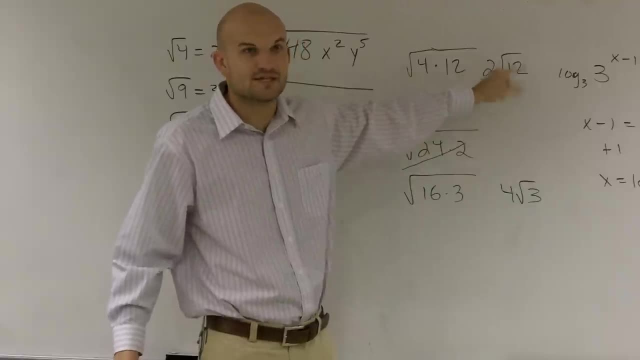 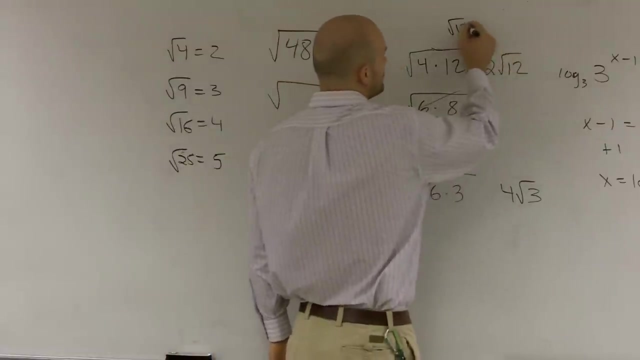 wrong with this one. But what you notice is: you can do this, you can simplify this one again. So it's not wrong, it's just you need to simplify it again. So square root: now you can do square root of 12, can reduce down to 4 times square root. 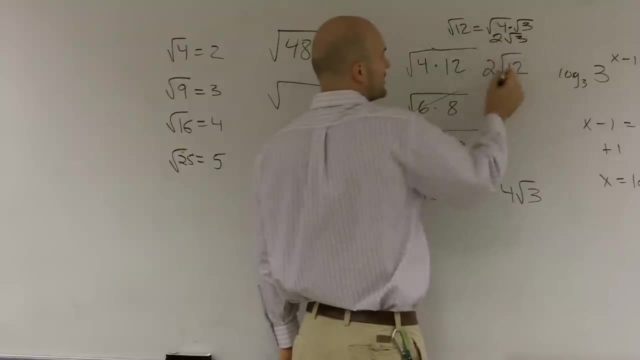 of 3.. Which that becomes 2 radical 3, right, And then there's automatically already a 2 there, so you'd still get 4 radical 3.. Oh, Do you see the difference? Yeah, So there's nothing wrong with choosing that. just try to always choose the largest number. 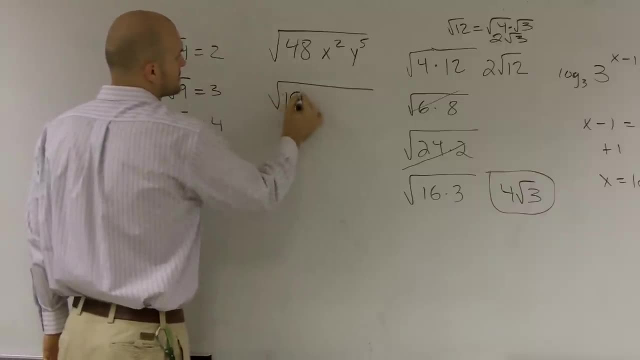 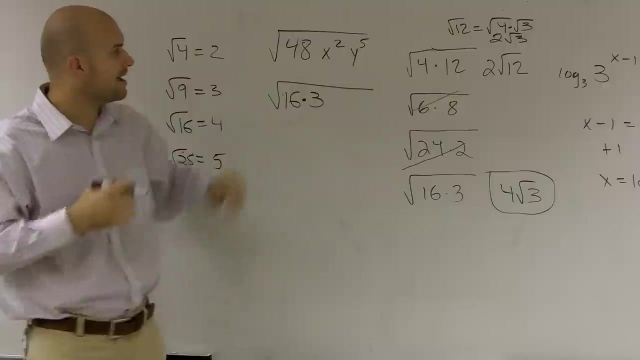 So, So you can add 16 times 3,. now, when you're dealing with numbers, with exponents, that's a little bit different, Alright. And the reason why is: um, you guys should know that square root of x, squared is just: 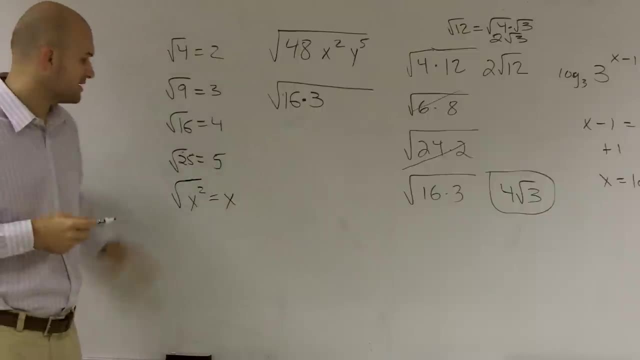 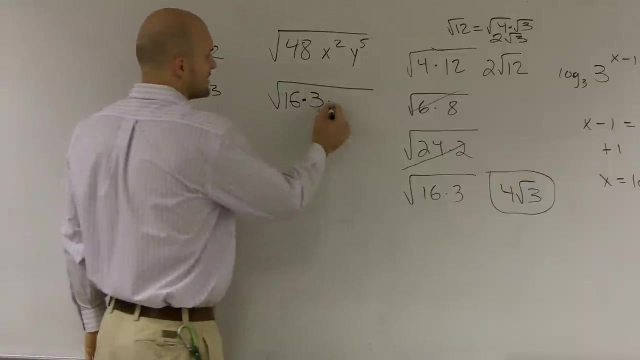 going to equal x, right? So what we want to do is we want to see if we can pair these as many squares as we possibly can. So what I can write this, as you know: x squared- y squared times- y squared times- x squared. 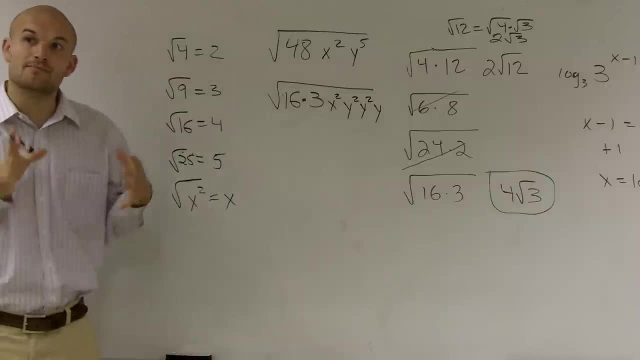 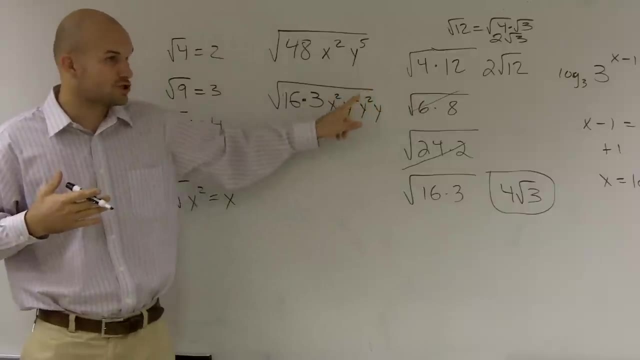 y squared times y squared times y squared. Why is there that extra y there? Remember, when you're multiplying exponents, you- I'm sorry- when you're multiplying numbers with exponents, you're adding the exponents. So this is 2 plus 2 plus 1.. 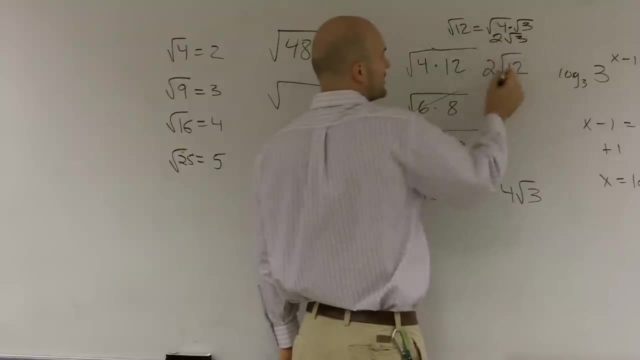 of 3.. Which that becomes 2 radical 3, right, And then there's automatically already a 2 there, so you'd still get 4 radical 3.. Oh, Do you see the difference? Yeah, So there's nothing wrong with choosing that. just try to always choose the largest number. 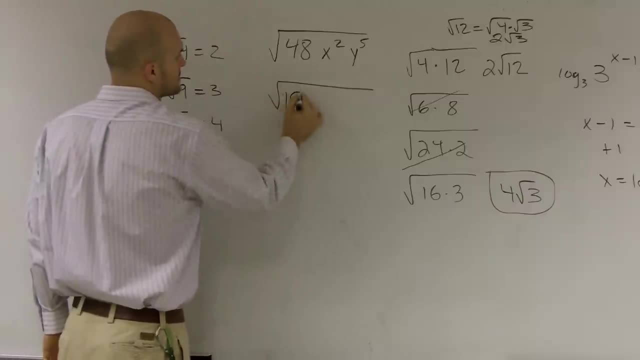 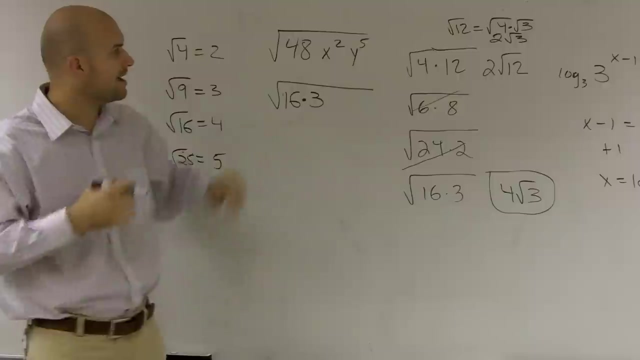 So So you add 16 times 3,. now, when you're dealing with numbers, with exponents, that's a little bit different, Alright, And the reason why is: um, you guys should know that square root of x, squared is just: 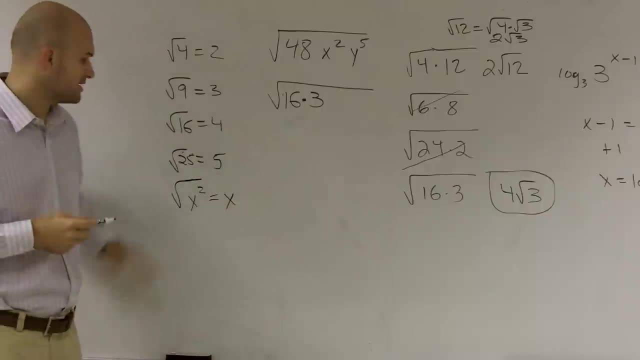 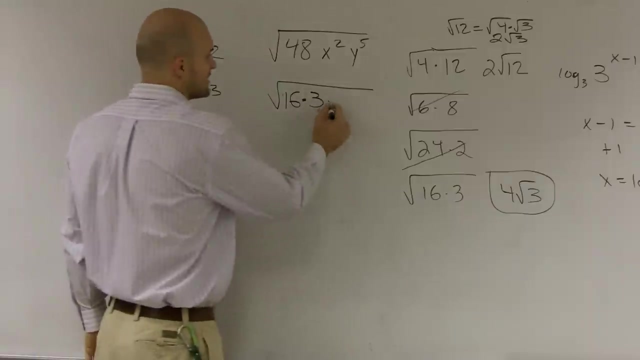 going to equal x, right? So what we want to do is we want to see if we can pair these in it as as many squares as we possibly can. So what I can write this: as you know: x squared, y squared times, y squared times, x squared. 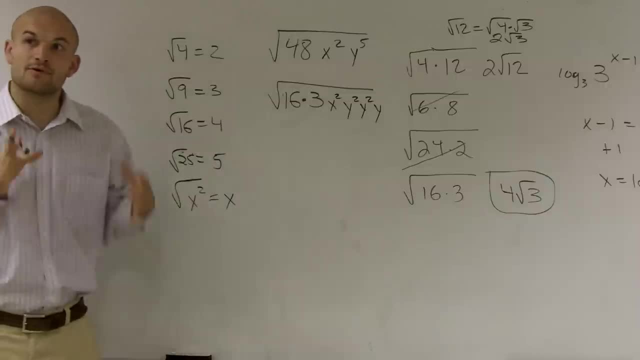 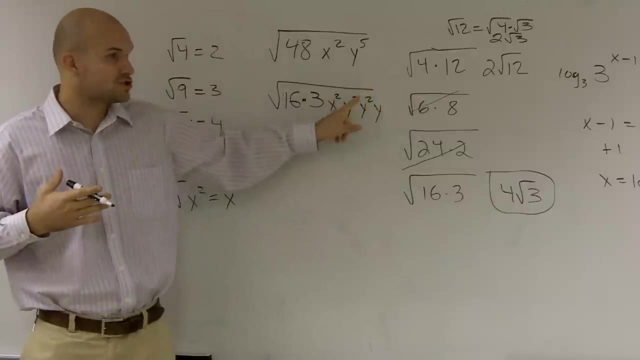 y squared times y and y. is there that extra y there? Remember, when you're multiplying exponents, you- I'm sorry- when you're multiplying numbers with exponents, you're adding the exponents. So this is 2 plus 2 plus 1.. 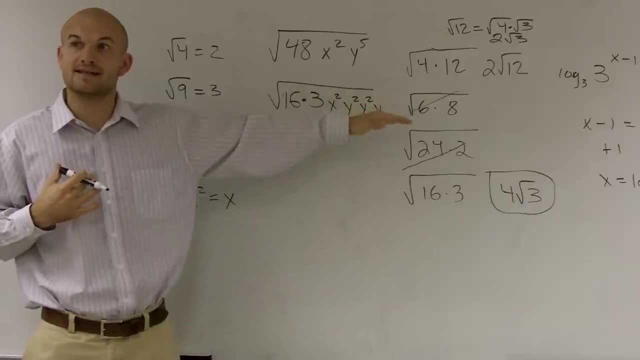 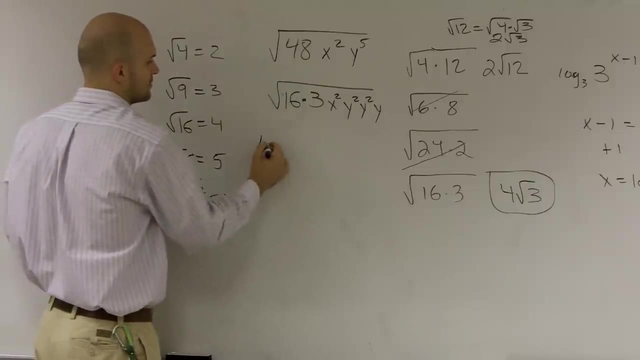 Right. Remember the properties of exponents. When you multiply, you add the exponents. So that's how I'm, that's why I separate this one a little bit differently. Well, the square root of 16 is obviously 4.. This becomes x times y times y, right? 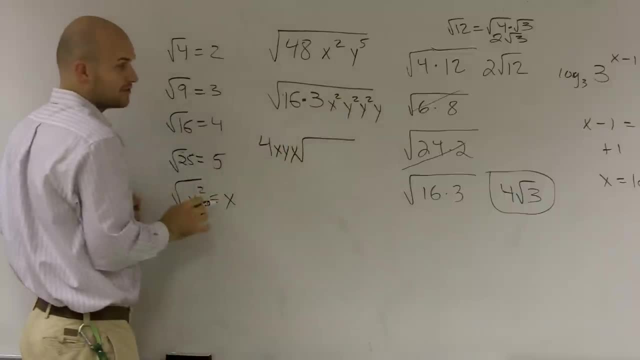 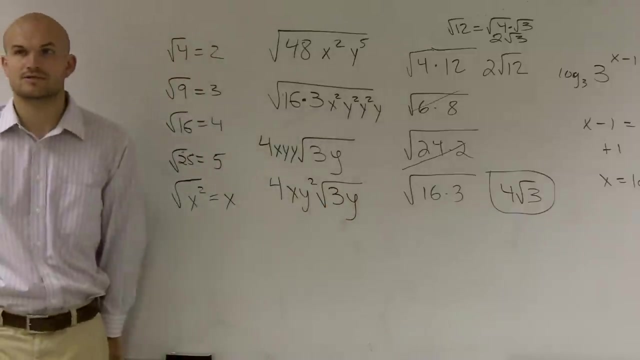 Because it's x squared Right, Because those both cancel out to give you your single variable. so you're left with a 3y. So it wouldn't be xy squared Yep. So then your final answer is 4xy squared times the square root of 3y. 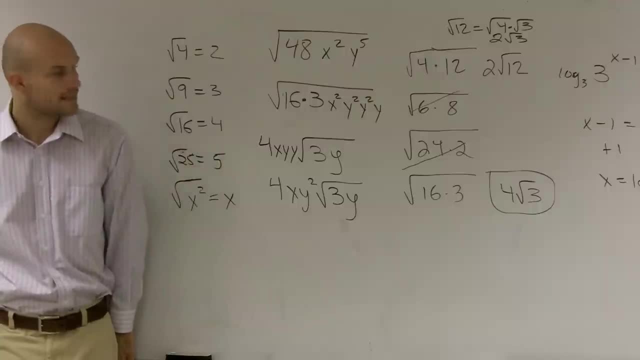 Questions on this. Yes, Why don't you use 4 times 12?? But it's the same thing. just, you have another step together. I'll pull out the video and I'll show you. You just have to assemble that, Okay. 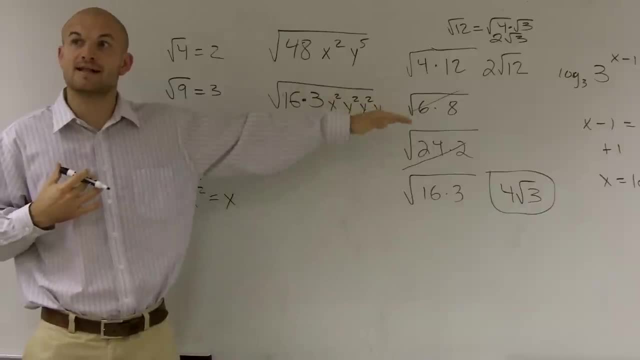 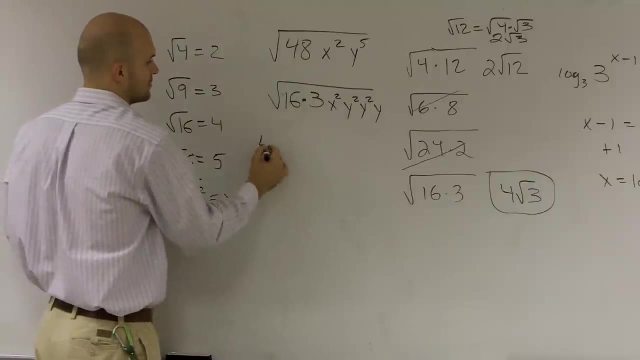 Right, Remember the properties of exponents. When you multiply, you add the exponents. So that's how I'm. that's why I separate this one a little bit differently. Well, the square root of 16 is obviously 4.. 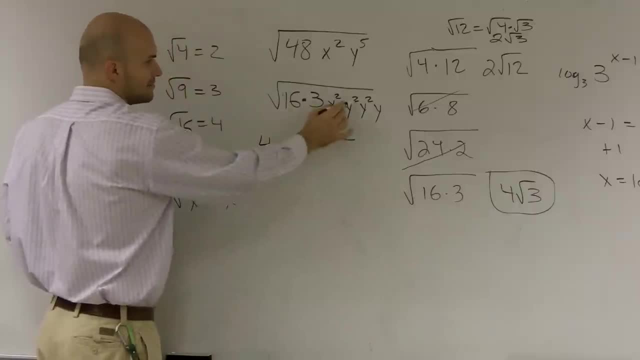 This becomes x times y times y, Right, Because those both cancel out to give you your single variable. so you're left with a 3y. So it wouldn't be xy squared Yep. So then your final answer is 4xy squared times the square root of 3y. 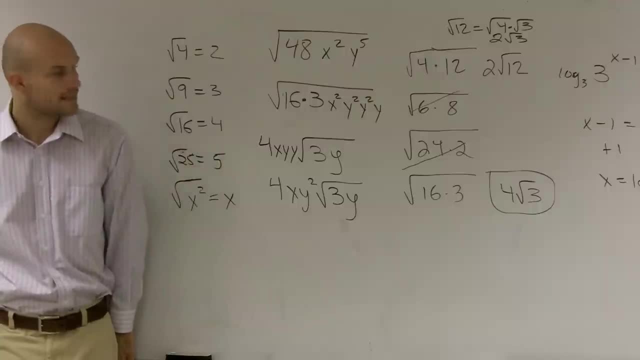 Questions on this. Yes, Why did you use 4 times 12?? Because it's the same thing. just, you have another step to go. I'll pull up the video and I'll show you. You just have to assemble that, Okay. 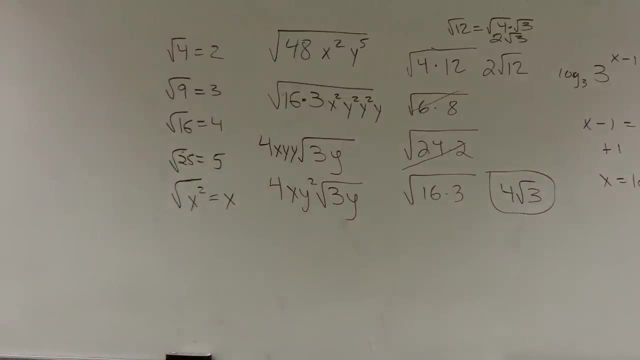